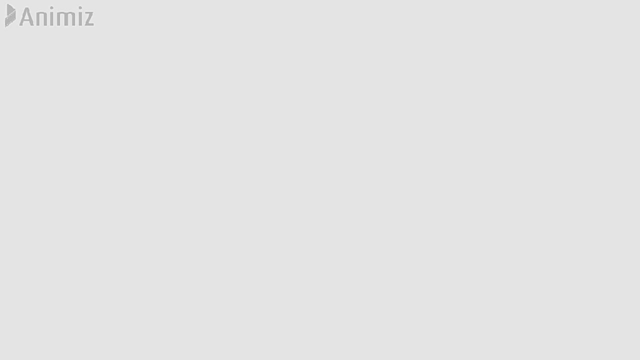 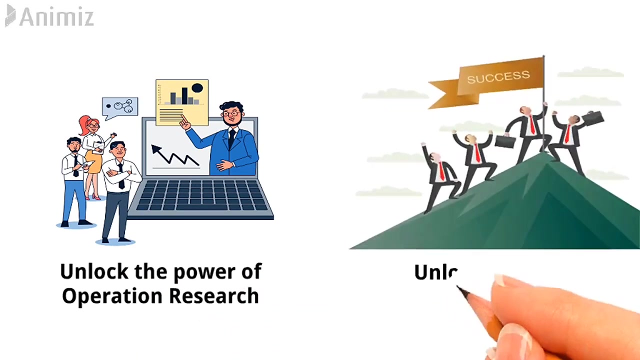 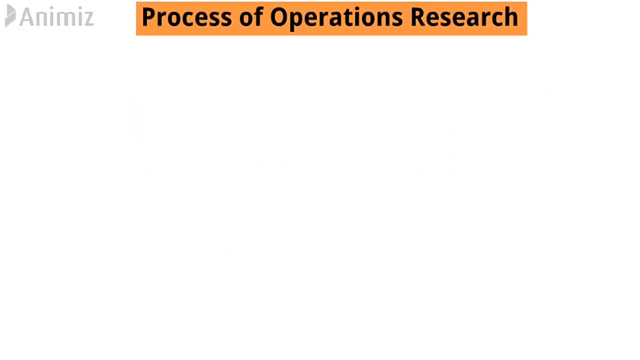 to managing financial risks. operation research is revolutionizing the way organizations operate. Unlock the power of operation research for your business and unlock a world of possibilities. The process of operations research can be broadly broken down into the following steps: Step 1. Identifying a problem that needs to be solved. 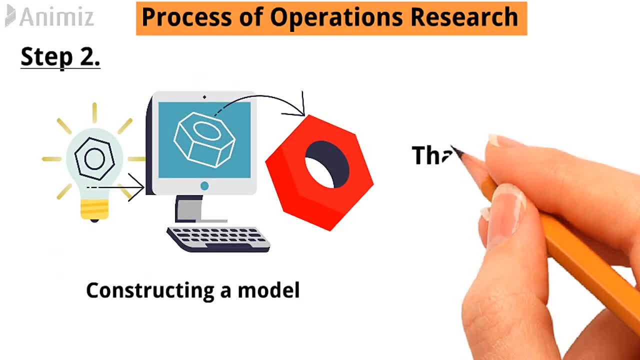 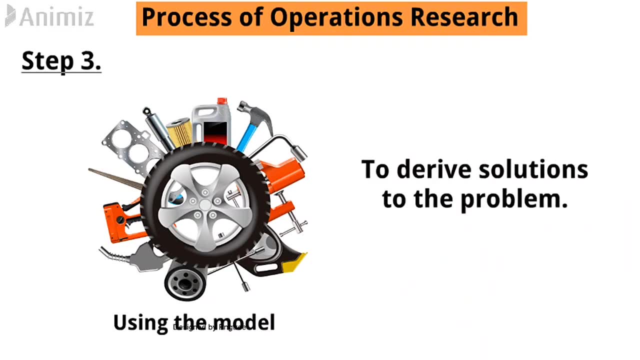 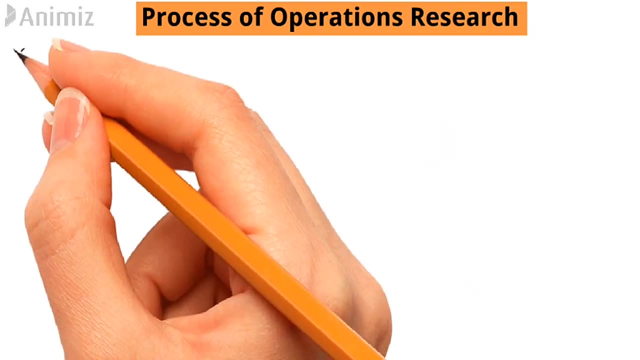 Step 2. Constructing a model around the problem that resembles the real world and variables. Step 3. Using the model to derive solutions to the problem. Step 4. Testing each solution on the model and analyzing its success. Step 5. Implementing the solution to the actual problem. 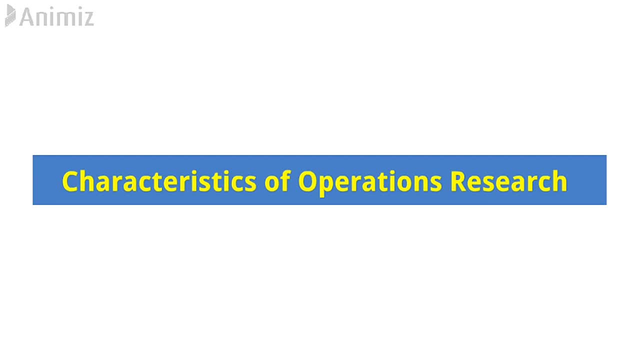 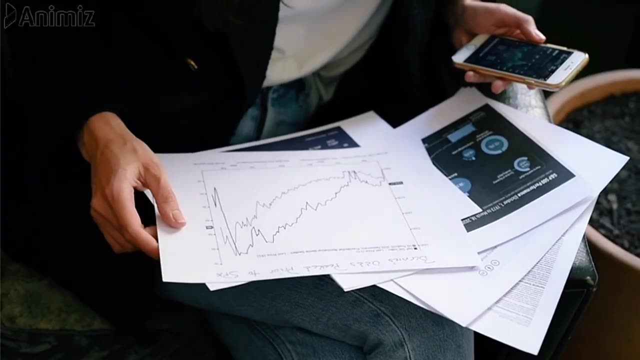 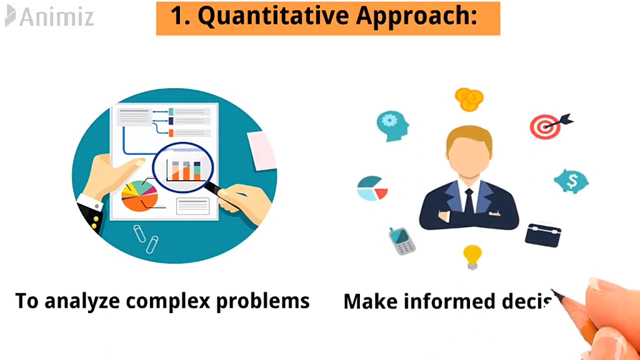 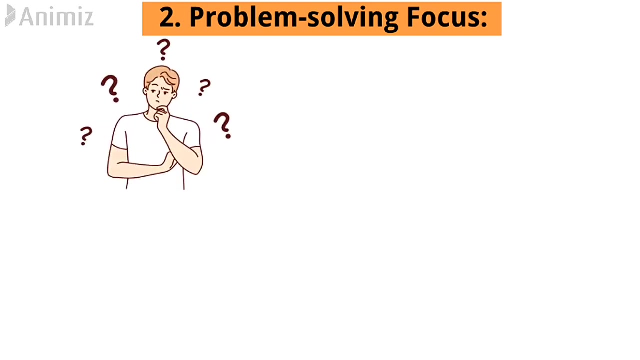 Characteristics of operations research. Let's discuss some key characteristics of operations research. 1. Quantitative approach: Operations research emphasizes the use of mathematical modeling and quantitative techniques to analyze complex problems and make informed decisions. 2. Problem-solving focus: It involves identifying the key problem areas. 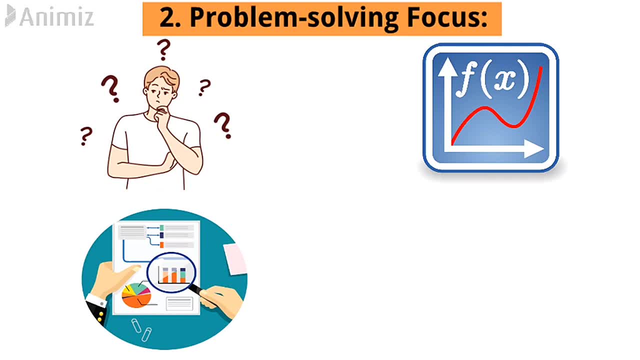 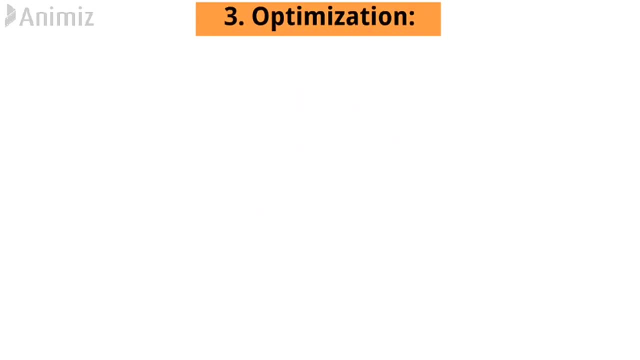 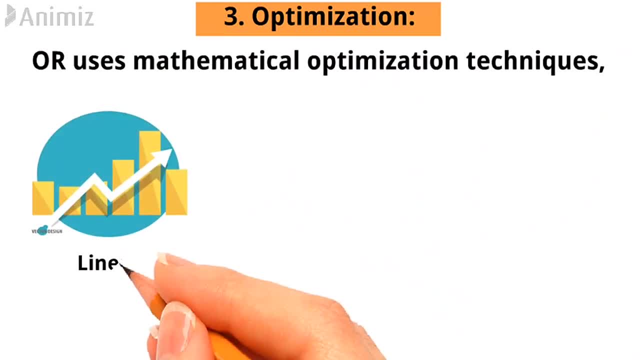 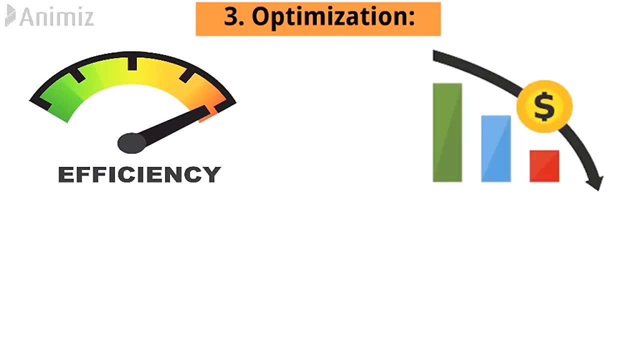 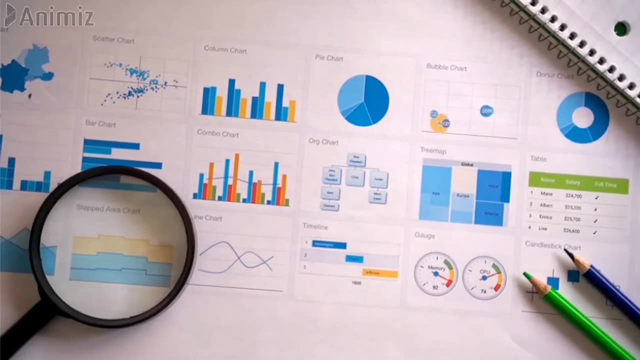 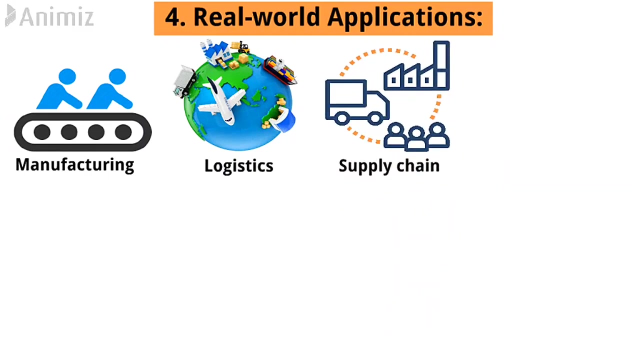 Optimization is a fundamental concept in OR R. uses mathematical optimization techniques such as linear programming, integer programming and nonlinear programming to maximize efficiency, minimize costs or achieve other desired objectives. 4. Real-World Applications: Operations research finds applications in diverse sectors including manufacturing, logistics, supply chain management, transportation, healthcare, finance, telecommunications and energy. 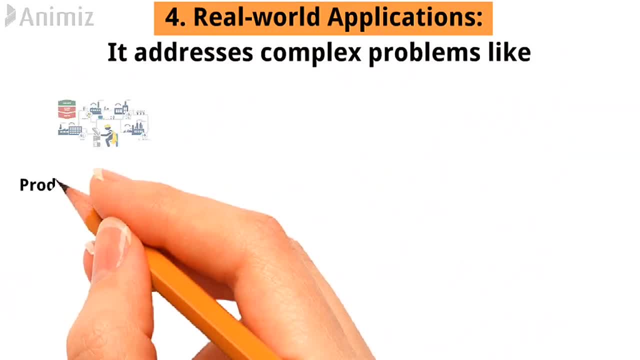 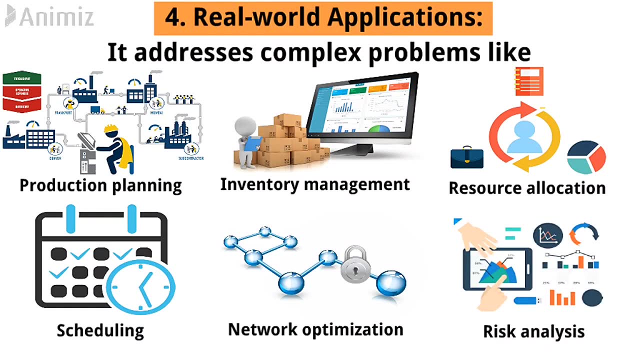 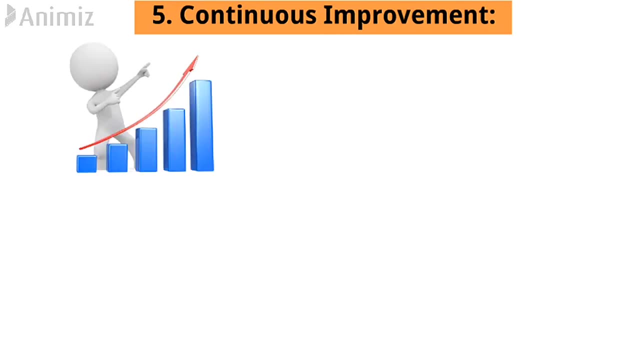 It addresses complex problems like production planning, inventory management, resource allocation, scheduling, network optimization and risk analysis. 5. Continuous Improvement: Operations research promotes a culture of continuous improvement by developing models that can be updated and refined as new information becomes available.